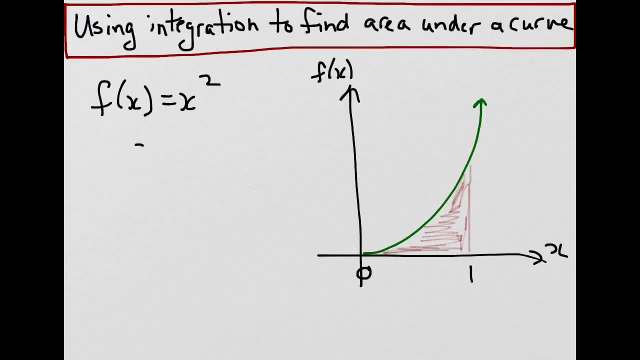 of calculus, which tells us that if we integrate our function x, squared with respect to x from 0 to 1, this will equal the area under the curve. This tells us, applying the fundamental theorem of calculus, that we need to find the antiderivative. 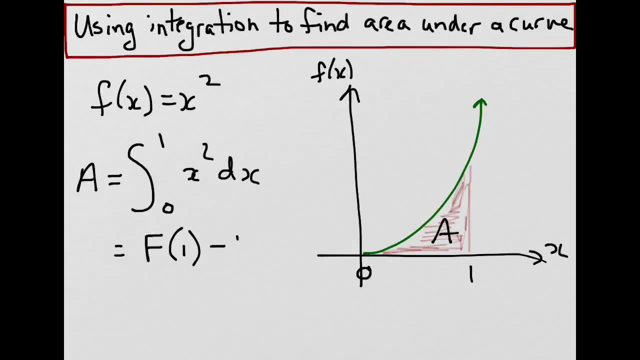 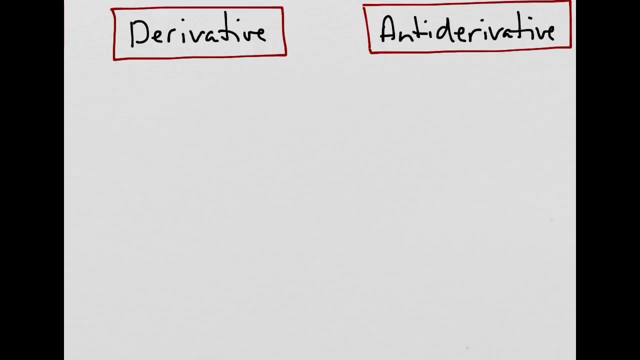 of f of x at 1, and subtract from that the antiderivative of f of x at 0. So how do we find the antiderivative? Well, let's go over to the side here and just review a couple of concepts. 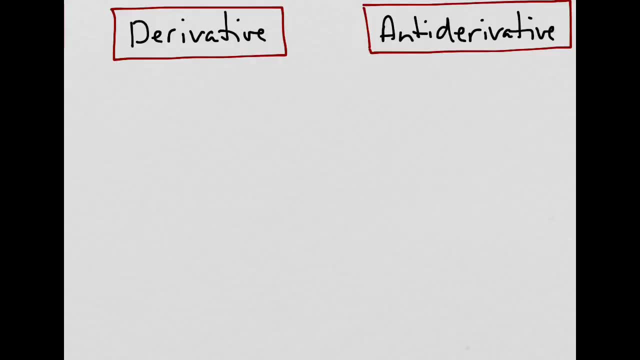 The derivative and the antiderivative can be thought of as opposites of each other. So let's say we had a function f of x equals x squared. We know that if we were going to find the derivative of this function, it would equal. 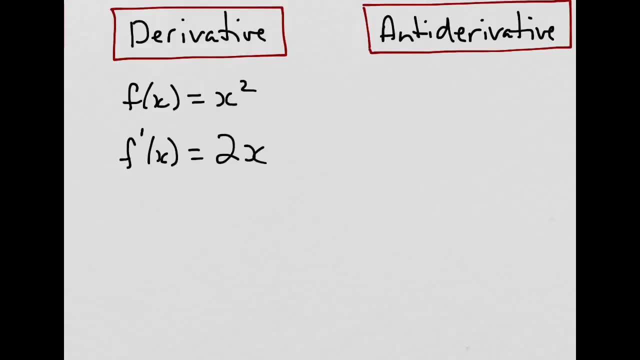 2x. The power rule tells us to take the exponent, multiply it by what's in front and then subtract 1 from the exponent. So if we had the same function- f of x equals x squared- and wanted to find the antiderivative, 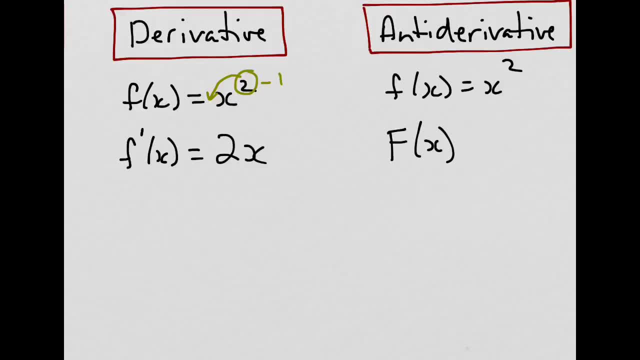 of this function, we'd do the exact opposite. We would add 1 to the exponent first, then divide by this value. So if we had the same function- f of x equals x squared- and wanted to find the antiderivative of this function, we'd do the exact opposite. 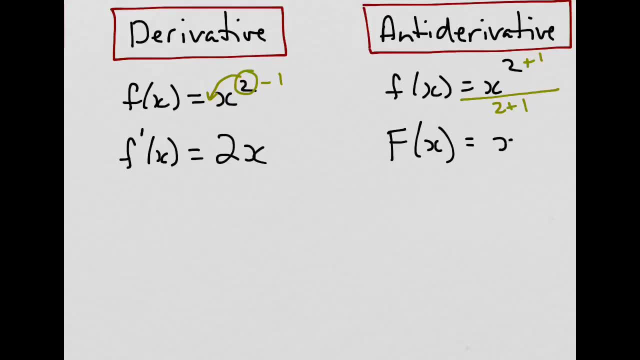 And this would leave us then with x cubed divided by 3, which becomes the antiderivative of x squared. We end up with a progression. So you have the function x squared and its derivative becomes 2x and then its antiderivative. 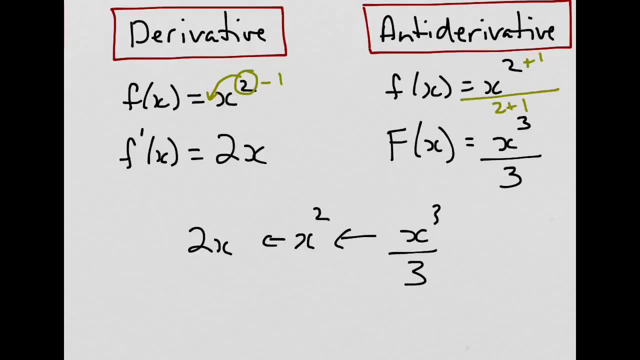 becomes x cubed over 3.. Such that the derivative of the antiderivative becomes x squared over 3.. So we end up with a progression: The antiderivative of the capital F function is the small f function, and the derivative of the small f function is the f primed of x function.